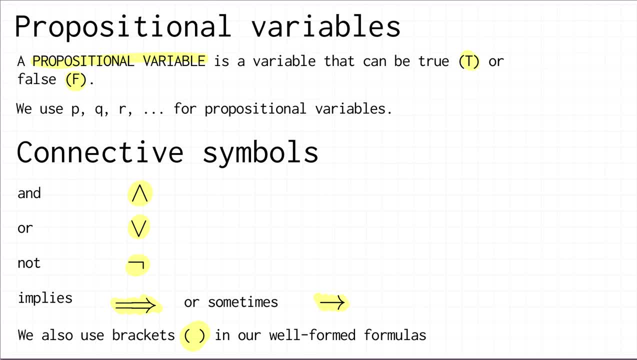 Okay, so a well-formed formula is not just any collection of propositional variable symbols, connective symbols and brackets. You have to obey some rules in order to make sure that what you have is a meaningful logical expression. 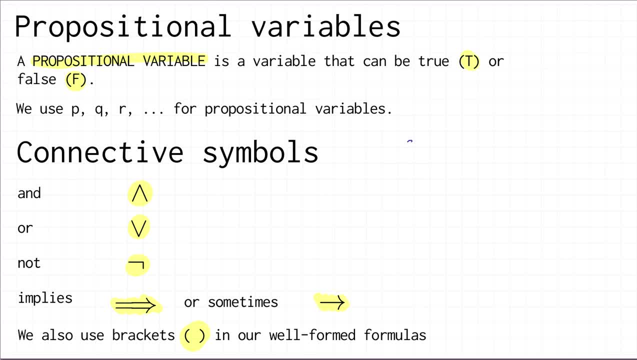 It's a bit like what happens in natural languages, right? There are lots of English letters A B C and so on, one up to z but not all combinations of those letters makes a legitimate word like if you have b x v y y z as far as i know that is not a meaningful english word so we have some rules 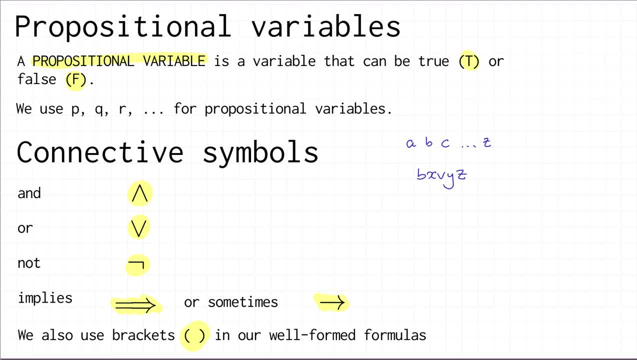 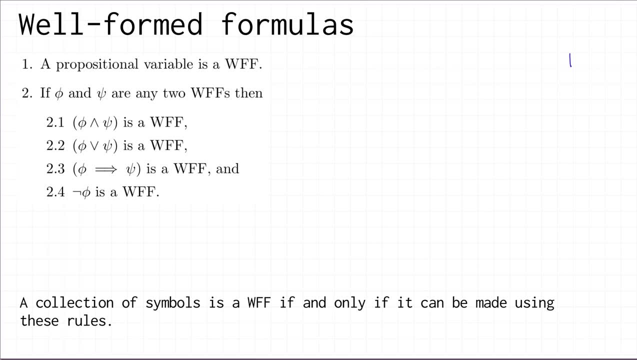 which tell us which collections of these symbols make a formula to which we can give a logical meaning and those rules are on this slide so we're going to define on this slide exactly what is and what isn't a well-formed formula and we do that using two rules so the first rule says that a 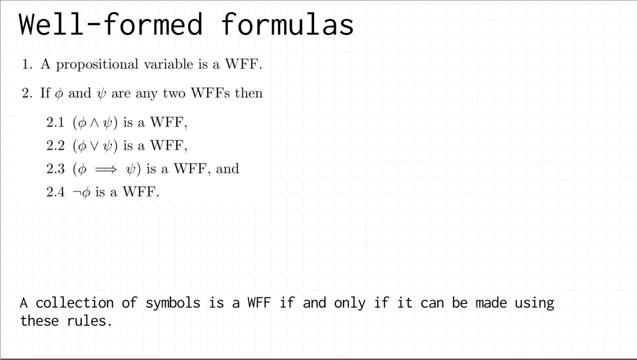 propositional variable on its own is a well-formed formula and the second rule is that if you have two well-formed formulas phi and psi then brackets phi and symbol psi close brackets is a well-formed formula that's rule one or 2.1 or 2.2 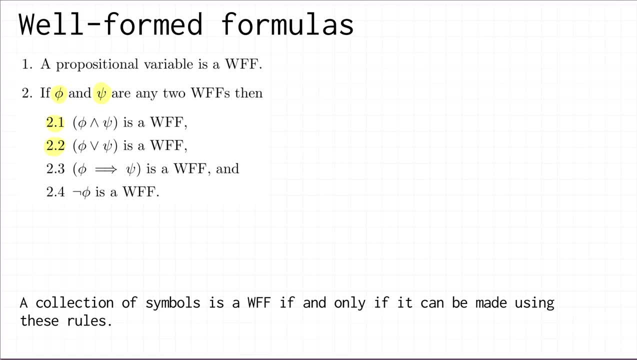 is that brackets phi or symbol psi close brackets is a well-formed formula 2.3 says that brackets phi implies psi close brackets is a well-formed formula and rule 4 says that not phi is a well-formed 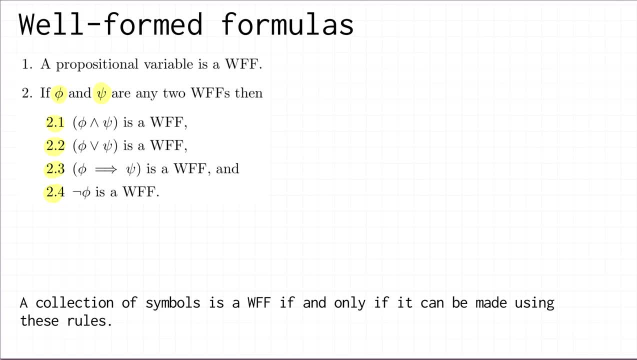 formula the idea is that a collection of symbols is a well-formed formula if and only if you can make it using these rules so if you can make something using this rules it's a well-formed formula 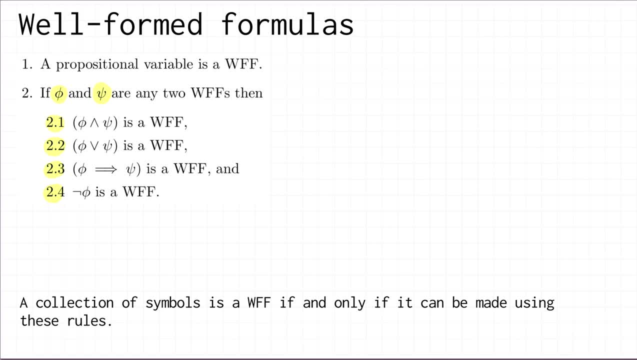 something is a well-formed formula then you must be able to make it using these 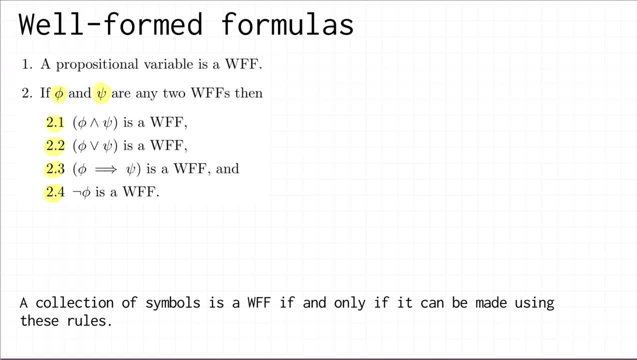 rules so let's look at an example then of a well-formed formula so let's just take some propositional variables first of all so we'll let P and Q be 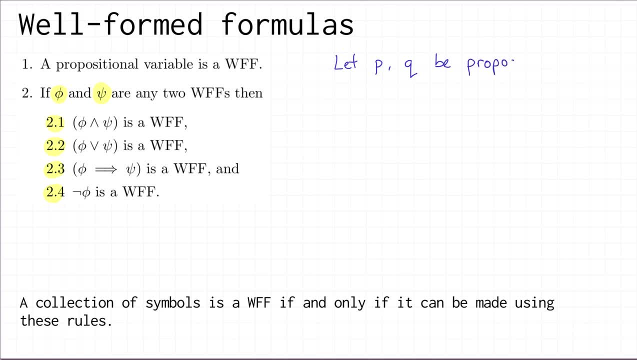 propositional variables then P is a well-formed formula okay that's rule one 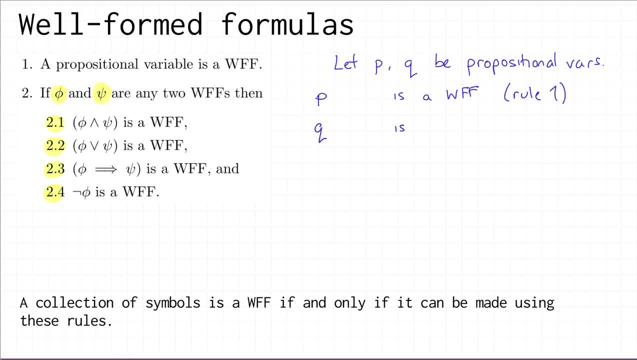 Q on its own is a well-formed formula and again that follows because of rule one 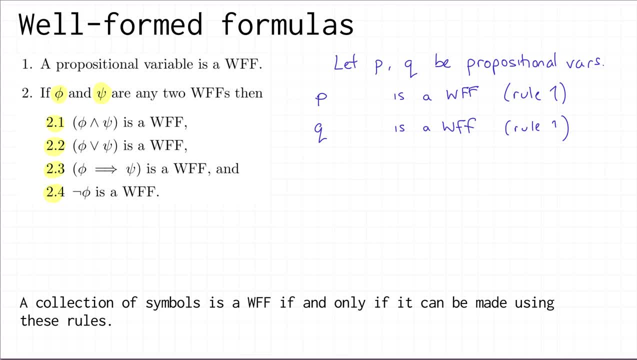 okay now we can do something more interesting we know that these two things are well-formed formulas and we know that by rule 2.1 whenever you have brackets and then a well-formed formula 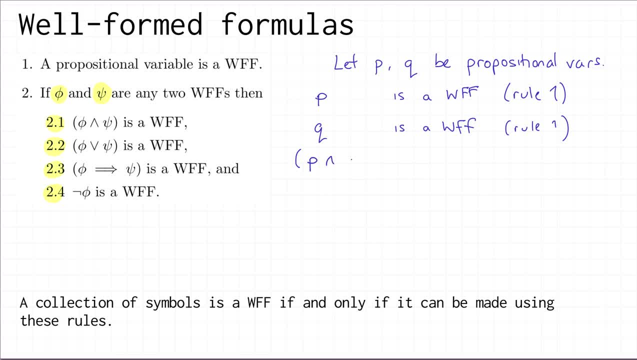 and then and and then another well-formed formula and then close brackets that is a well-formed formula so that is by rule 2.1 so i should say that wff here always stands for 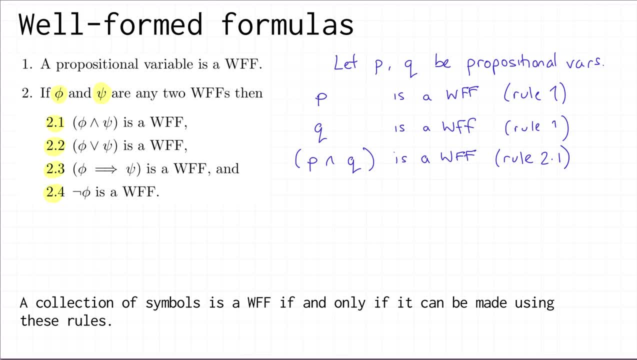 well-formed formula of course you guessed that okay so we can do even more complicated stuff now because we know that brackets p and q brackets is a well-formed formula we know that q is a 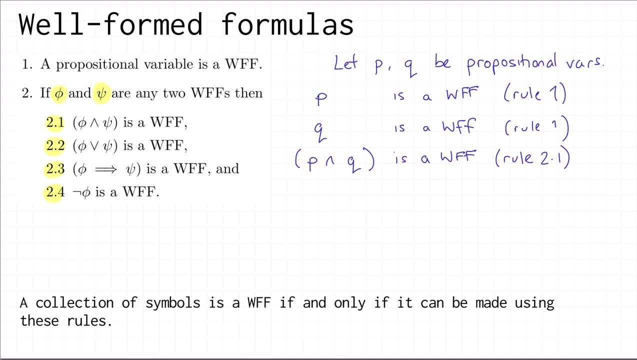 well-formed formula so let's use i don't know let's use 2.4 we haven't used 2.4 yet so not q would be you a well-formed formula okay that's rule 2.4 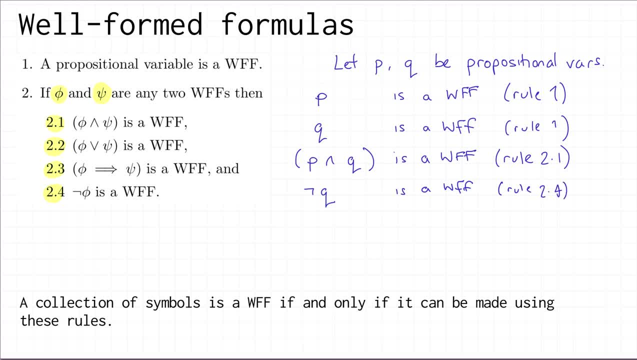 and finally let's do one more so if i now have brackets and then any well-formed formula we're going to use rule 2.3 here and then the implies symbol and then any other well-formed formula so we'll use this then that is a well-formed formula so we used 2.3 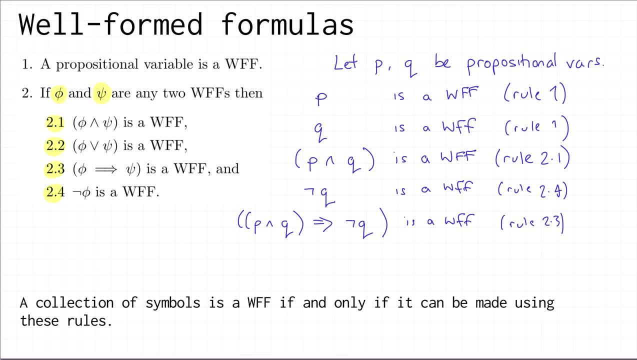 so this is how we build up complicated well-formed formulas by using the rules rule number one and rules 2.2 through to 2.4 repeatedly and again let me emphasize a collection of symbols is a well-formed formula if and only if you can make it using these rules 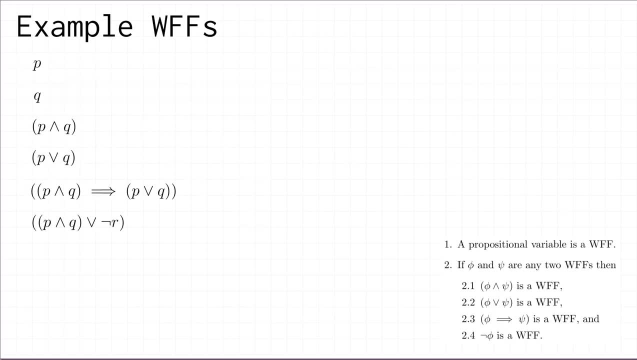 okay let's look at some more examples then so i'm going to repeat a little bit what i said before 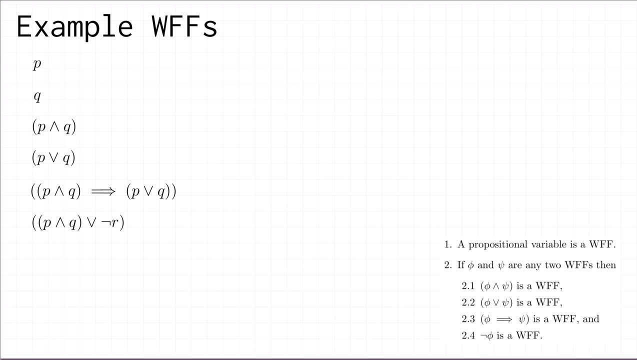 if we take p on its own so p is supposed to p and q are still propositional variables and this is a well-formed formula by rule one q is a well-formed formula by rule one